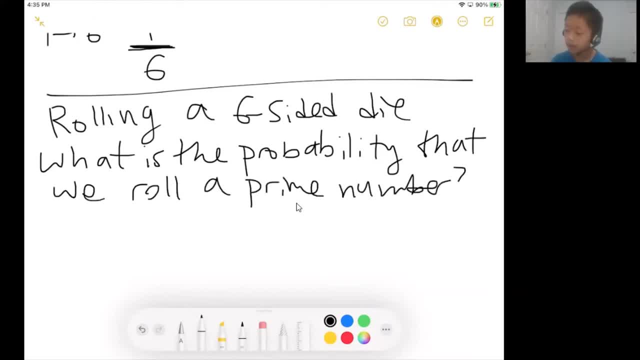 So, uh, this is another like um slightly more complicated but still not like too difficult, like common probability problem. So, again, what we want to do is we want to find the number of successful outcomes divided by the number of possible outcomes. So, um, here we see again. 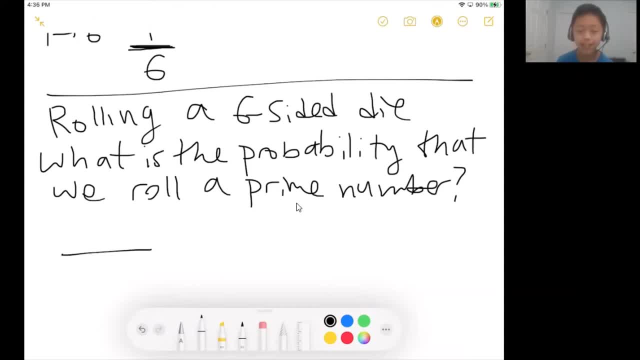 that the number of like possible outcomes. usually that's the easier one to calculate, like the, the, the denominator of the probability formula. So like there are six-sided die, numbered one, three, six, what is the probability that the number rolled is prime? 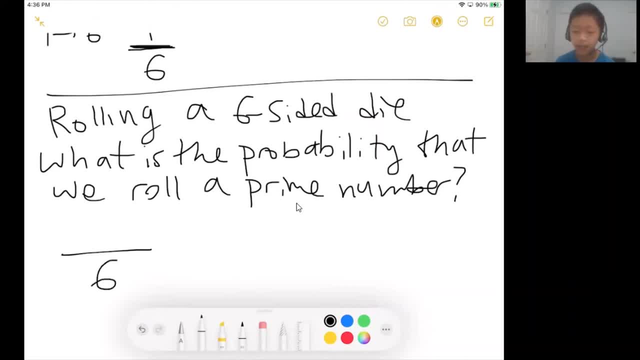 It's possible outcomes, because the die can land on any number from one through six. So now we need to count how many successful outcomes there are. So, uh, if we were to roll a prime number, we notice that the only prime numbers from one through six are two, three. 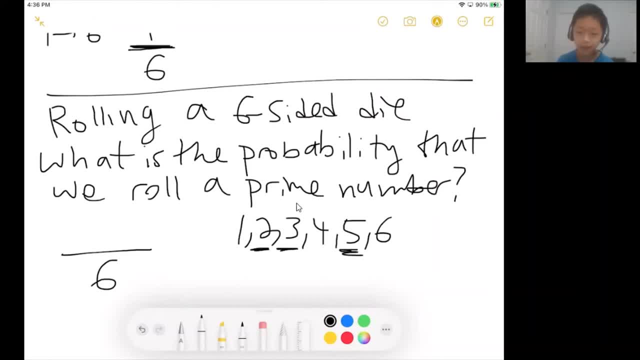 and five. So that's going to be, uh, three possible prime numbers. You would do like three divided by six and that would be just one half. So that means the probability, uh, of rolling a prime number would be one half. 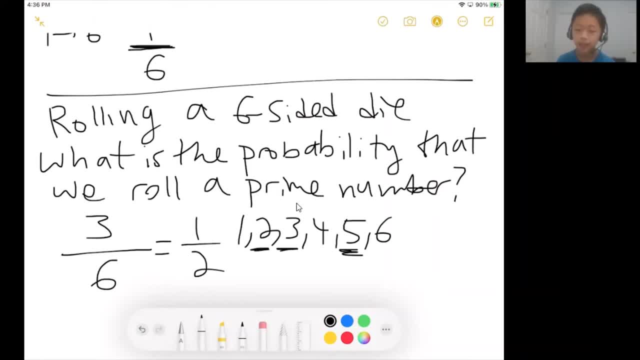 And I should also probably mention this- like what probability? like, as I've said already, like probability just represents the chances of something happening, But like of course it's. this doesn't mean like, um, it's going to, it's. this doesn't mean like it's guaranteed to be, like 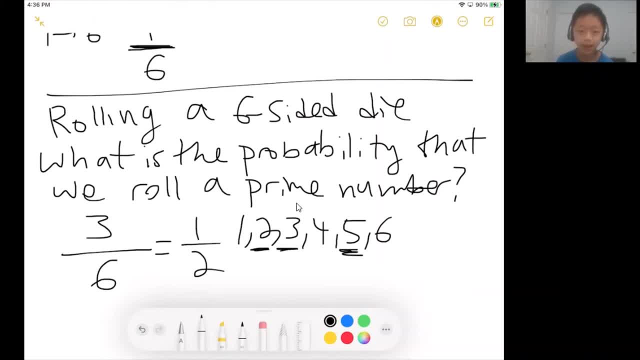 this Like, just because I roll a uh, a die, like 10 times, for example, doesn't mean exactly half of them will result in a prime number. Um, what it means is that, like, like, it's kind of this is: 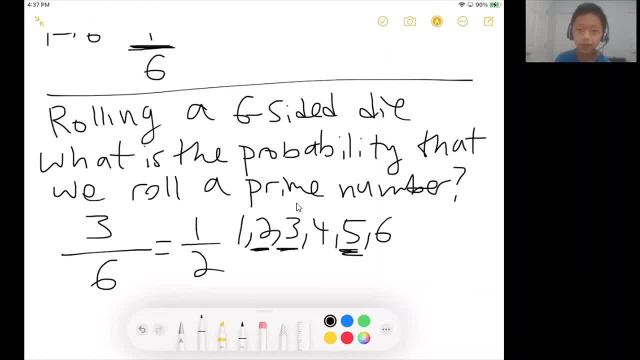 what we call like the theoretical probability, Like as you, uh, as you like. basically, what this means is, as you roll the die, like more and more times, like you roll it, like a hundred times or a thousand times, or 10,000 times, like the. 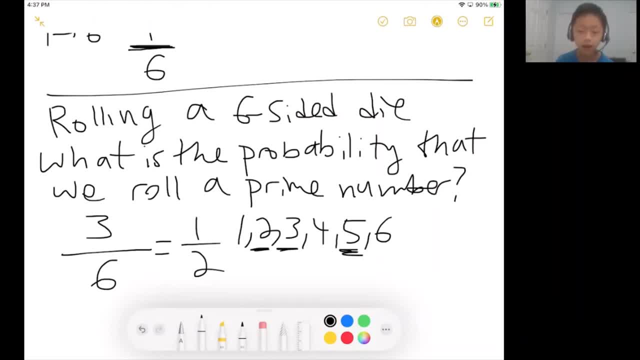 eventually, eventually, approximately half of these uh rolls are going to result in a prime number. So it's like it's like in the long run, like it's kind of like an approximation: um, how many of them, what proportion of them, are going to satisfy the condition?